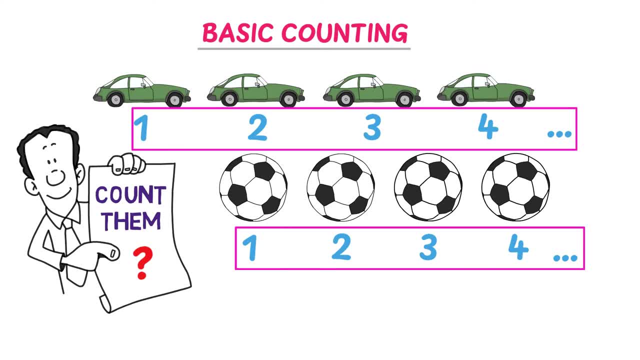 We start basic counting from one, two, three, four and so on, And mathematics we call all these numbers as natural numbers. So one, two, three, four and so on are all natural numbers because we use them for basic counting, The set of natural 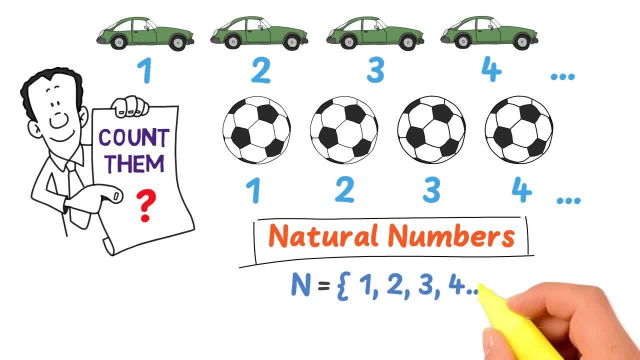 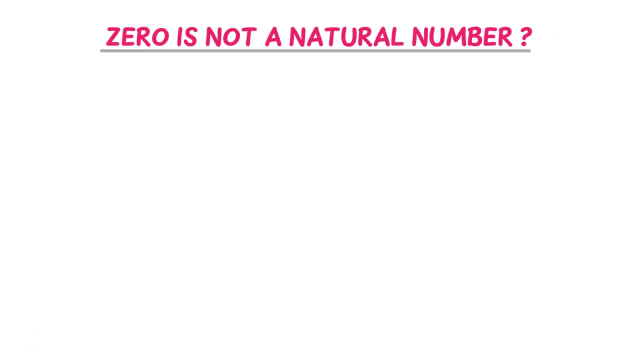 numbers is denoted by n, and it is equal to one, two, three, four and so on. Thus, remember that all basic counting numbers are called natural numbers. Now, why zero is not a natural number? Well, consider these bicycles. Let me again ask you to count them. 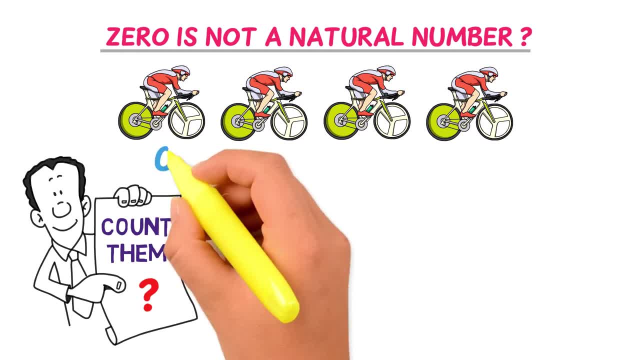 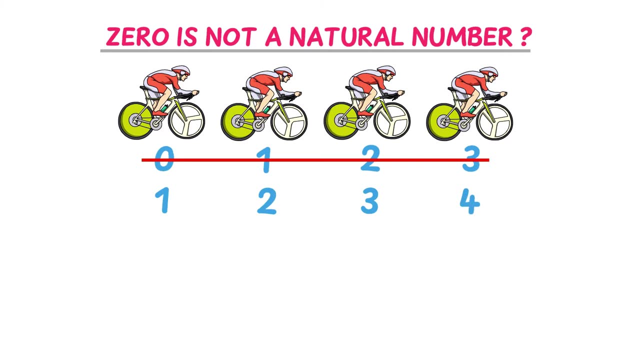 If you start counting these bicycles as zero, one, two and three. We all know that this is the wrong method of counting. We do not start counting from zero, We start counting from one, two, three and four. So there are four bicycles, not three bicycles From this example. 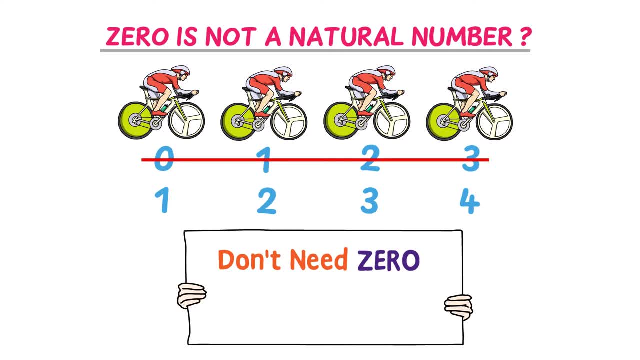 we learn that we do not need a use zero for basic counting. Therefore, it is not included in the set of natural numbers. While writing a set of natural numbers, n is equal to one, two, three, four and so on. Zero is therefore kicked out from the set of. 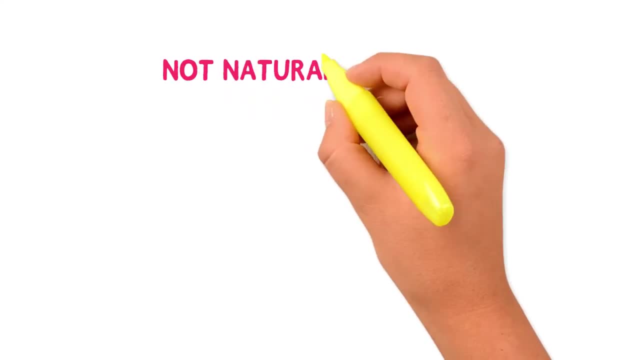 natural numbers. Finally, let me teach you that what numbers are not natural numbers? Well, the answer is very simple: All negative integers are not natural numbers, like minus two, minus nine, minus twenty, etc. Secondly, all decimal numbers are not natural numbers, like two point five. 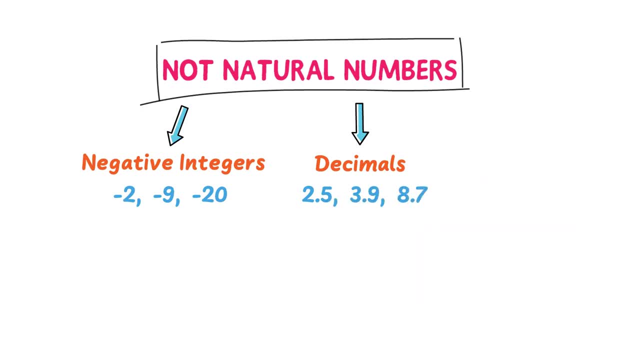 three point nine, eight point seven, etc. Thirdly, all fraction are numbers of p by q form are not natural numbers like two by three, one by six, etc. If you think that, why all these numbers are not natural numbers, then the answer is very simple. 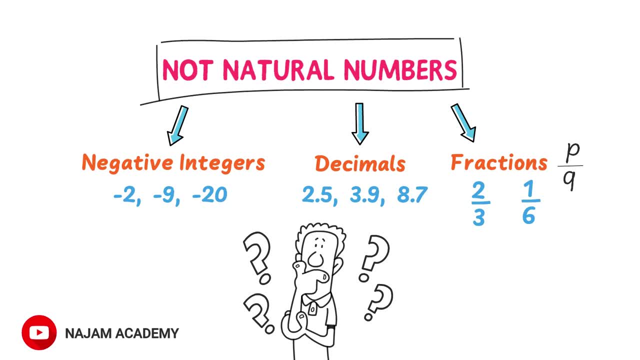 We do not use them for basic counting purposes. For example, we do not say minus two cars, two point five cars are two by three cars, etc. If you think that why all these numbers are not natural numbers, then the answer is very simple.